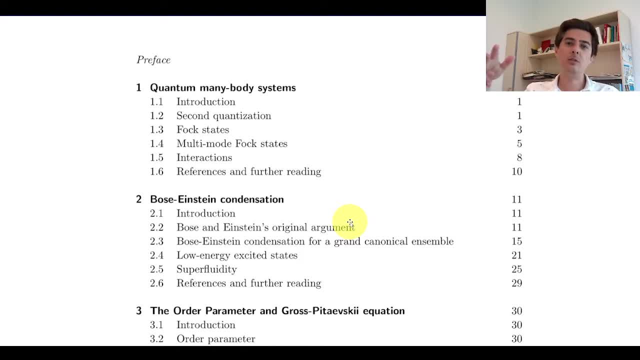 kind of phenomenon of Bose-Einstein condensation. This is when, if you start with a large, say gas of atoms and you start with a large say gas of atoms and you start with a large say gas of atoms, then all the gas of atoms they go into the ground state below some critical temperature, and so this: 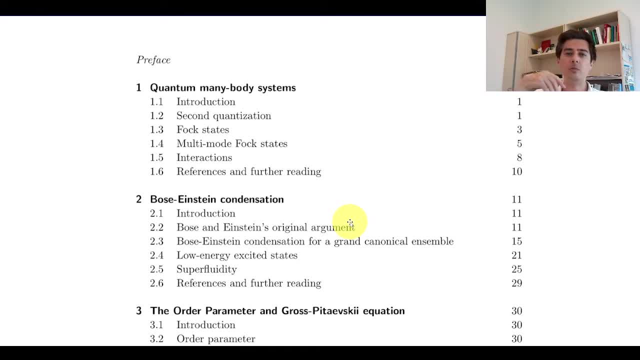 is some kind of phase transition which occurs, and this was originally predicted by Bose first, and then Einstein later saw Bose's result and kind of confirmed that this should happen, and so they're both credited for this, for this particular phenomenon. So I'm not quite sure exactly of the exact sort of you know exact. 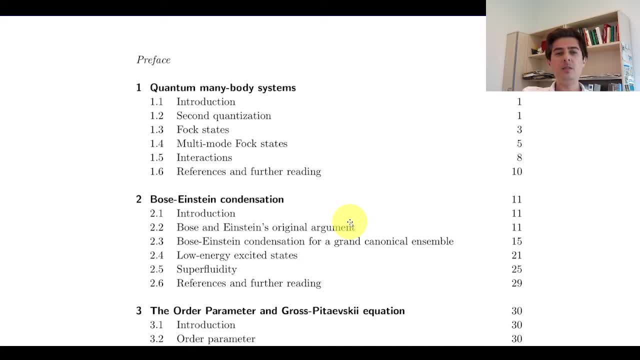 argument that Bose and Einstein presented, but at least this version is somewhat my interpretation and my understanding of their original argument. So, you know, if, if you find that you know this is not exactly what they said, then you know, please. you know, don't get too angry with me. I've embellished it for the purposes of what I think is a better way to kind. 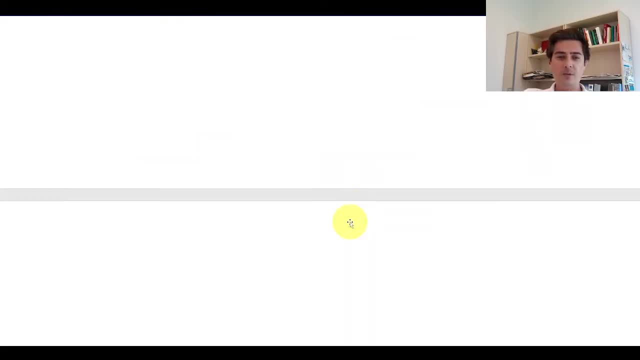 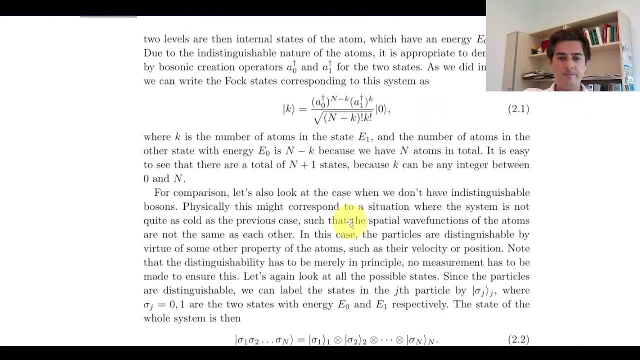 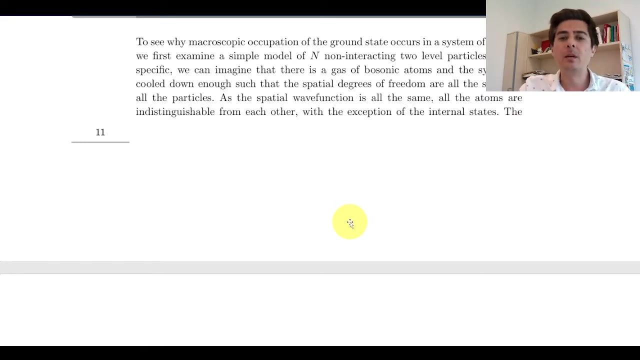 of understand this kind of argument in general. Okay, so let's have a look at this. So we're going to chapter two, Right, yeah, here we go, So in chapter two. so a good place to start with is to sort of understand a kind of prototypical system. So let's consider thinking about n non-interacting, two level. 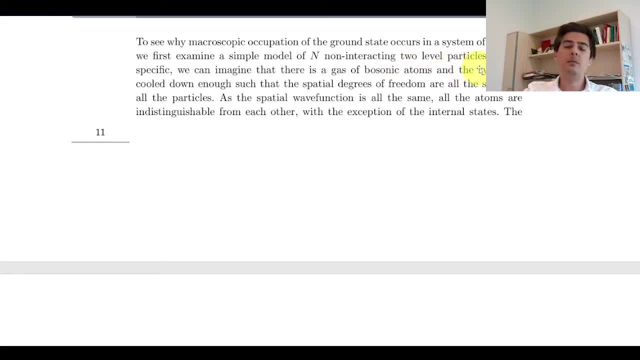 particles and you know, realistically, when you think about Bose-Einstein condensation, what you should probably really think about is some kind of, you know, say, container. It's containing a large number of atoms in it and these are all bosons. and then you cool the system down and spontaneously the system 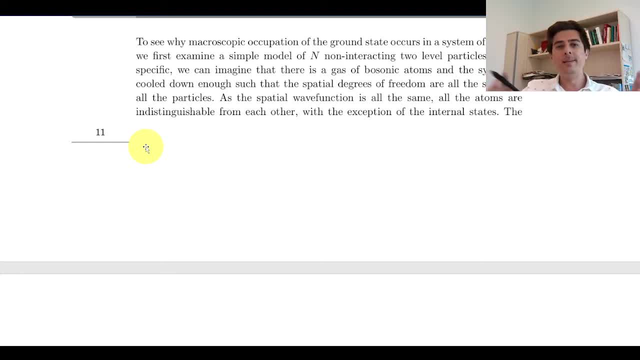 goes into the ground state, and the ground state would mean the ground state of the container that you are thinking about. So you know, if you, if you've got, you know some box here. what I mean by the ground state is, of course, so in a sort of idealized system. So here's our box, Then the ground. 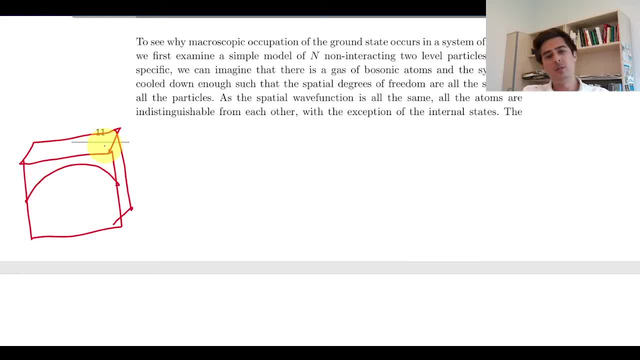 state would be some wave function which would be, just like you learn, in the infinite square. Well, the ground state should be some Gaussian looking shape, or maybe sine curve, or something like this. Right, So basically, what you'd say is that all these atoms are in this, in the same ground state, below a particular temperature. That's, that's basically the physics. 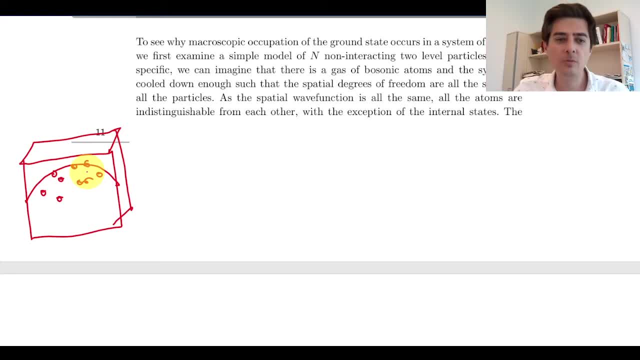 that we're looking for, But what we're going to do here is to not look at it so realistic. We're looking at a more sort of prototypical system, So what we're going to just consider is something a little bit simpler. So, instead of looking at all these motional degrees of freedom, we're going to just basically think of a bunch of, say, two. 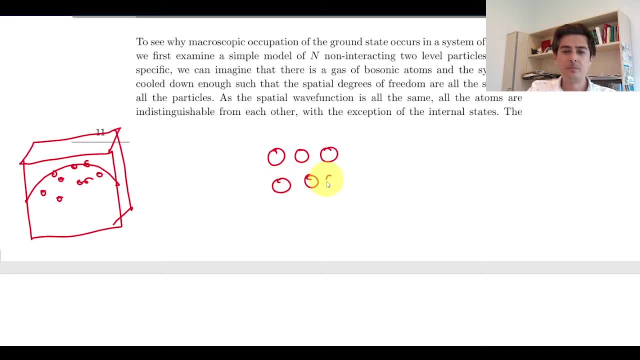 level atoms. So these are all, say, atoms. We're not really going to particularly worry so much about the actual motional degrees of freedom, as would be a little bit more realistic, Right? So we're going to consider a bunch of atoms and we're not not really, we're just 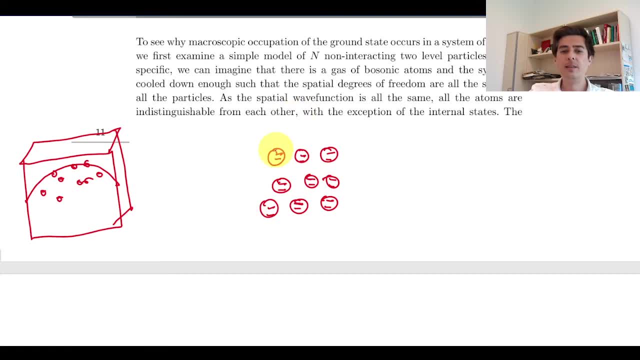 going to consider each of them to be some two level state, and there's an excited state for each atom and then there's a ground state for each one, And we're just basically going to look at the thermodynamics of this kind of kind of toy model, if you like. 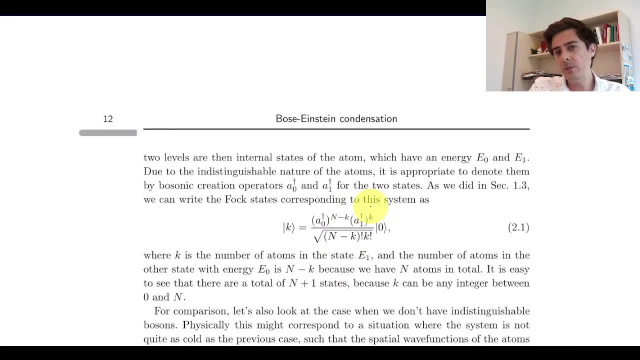 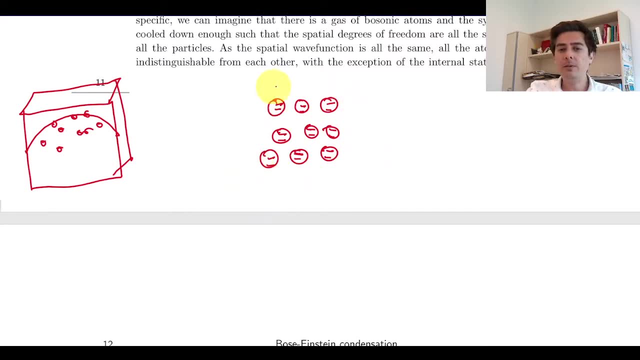 So So we can view these particles in two different ways. So we sort of have a choice of how we enumerate the states of the system, according to whether these particles happen to be distinguishable or indistinguishable. And what we're going to do is kind of contrast these two different cases and show that it gives really quite different results. 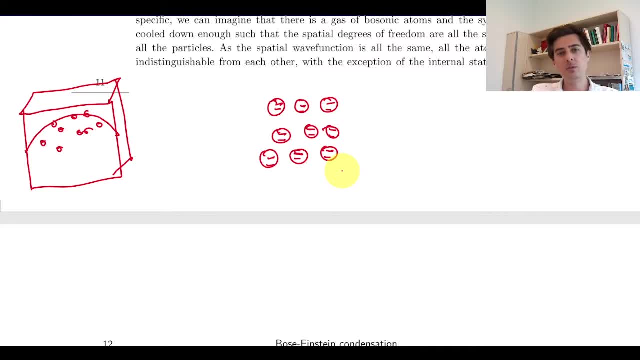 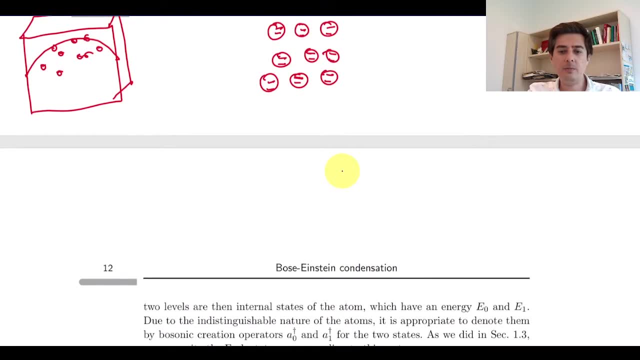 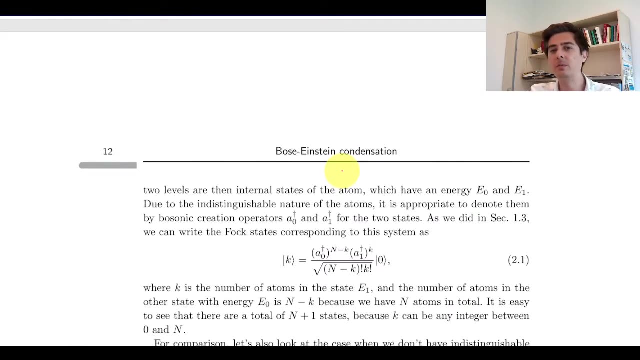 If you consider them to be indistinguishable, or if you consider them to be distinguishable, Right? So, firstly, if we consider the case of indistinguishable atoms. So this is a little bit more like what we started off doing in chapter one. 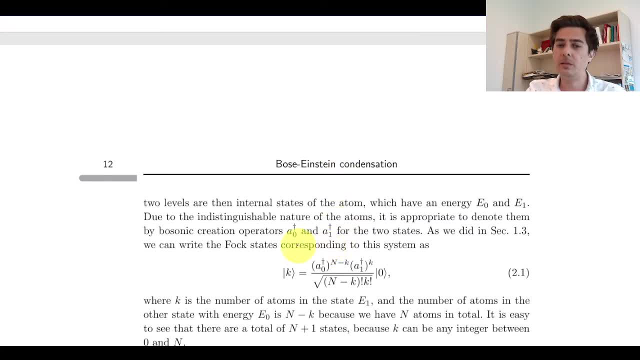 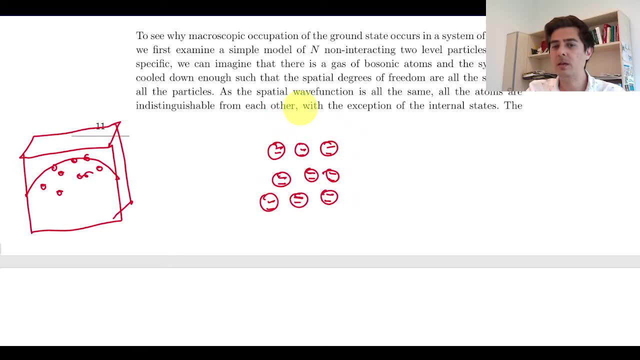 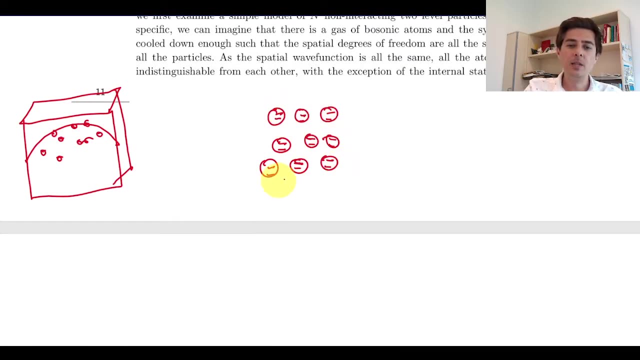 So we there wrote down all the kind of Fock states of a system And so because all these particles Are indistinguishable, Say you have got nine atoms and say you've got, you know, three in the excited state and then the other six in the ground state, like this: 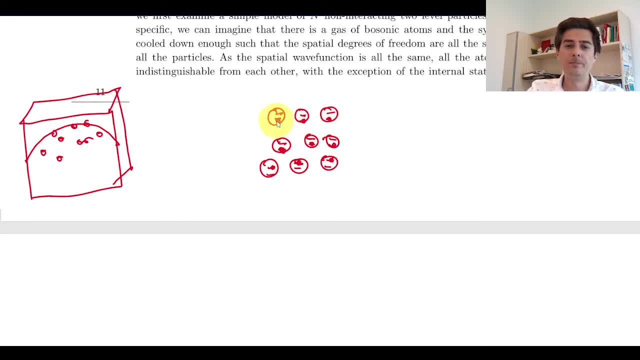 So six atoms in the ground state. Now, because these guys are all indistinguishable atoms, They're the only way that you Can really, And so are these, by the way. So these Between these three and between these six, they're all indistinguishable. 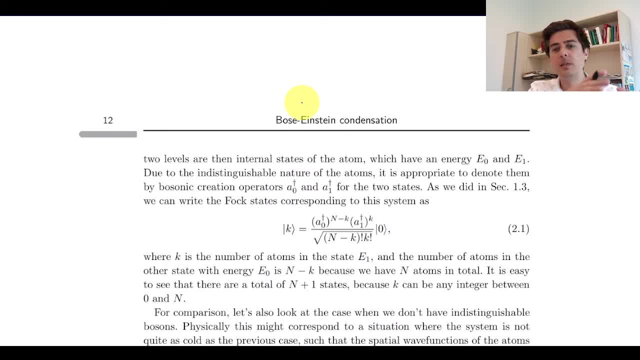 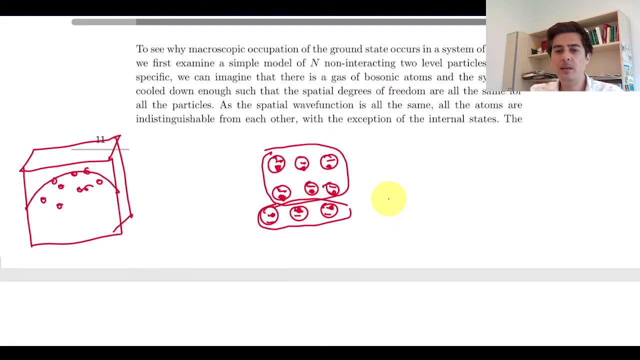 So really, the only way that we can enumerate the states of the system, using these bosonic operators that we learnt off in chapter one, And, And. so for this particular example, we would say we would write this particular state as A Fock state, where. 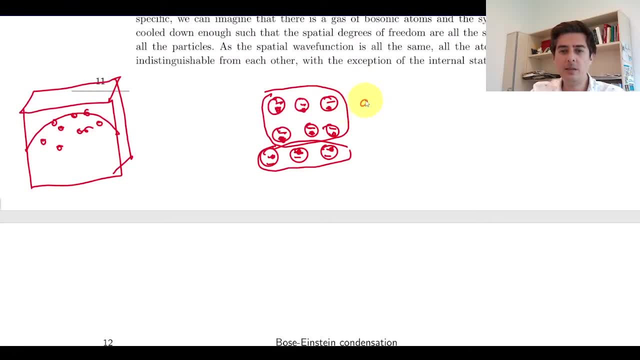 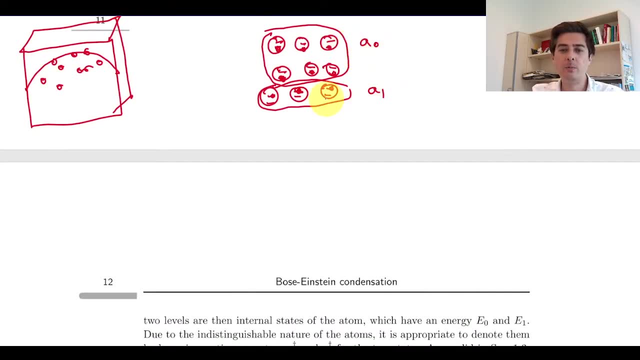 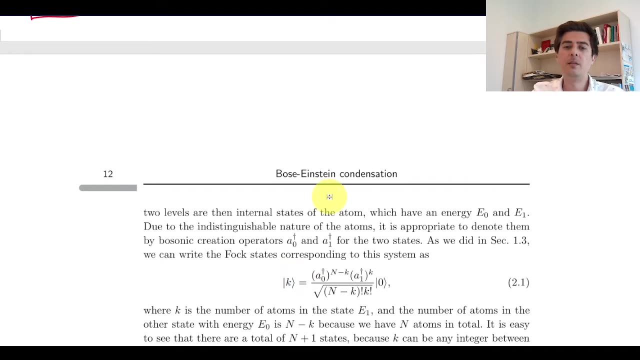 If we call these, these atoms here, these are the atoms, that which we're going to be labeling by a one and these atoms by- Sorry, a zero and a one, Then this would be: and if we call K, the number of atoms that are in the excited state. 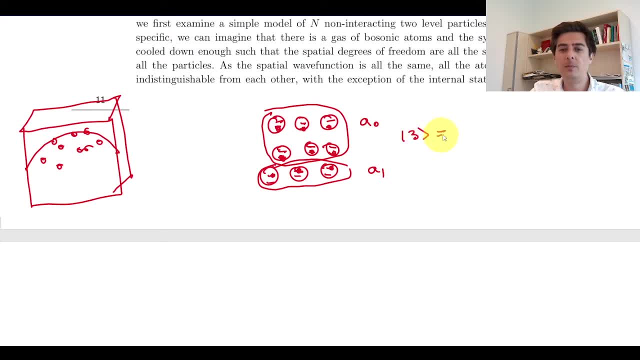 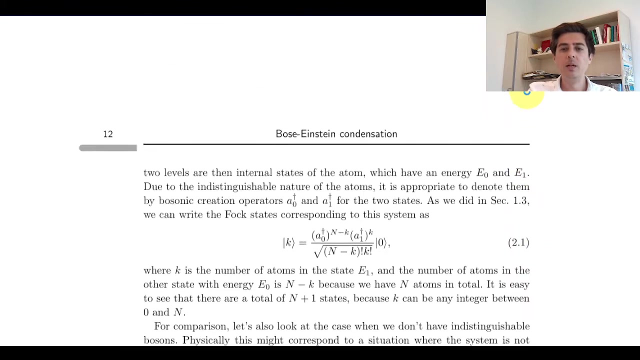 So there's three atoms in the excited state, So this will be Fock state number three, And that Means Actually There's six a zeroes and three a ones, and then we need these proper normalization factors like this- So that's how we would write it- for indistinguishable particles. but what if we had the same situation? 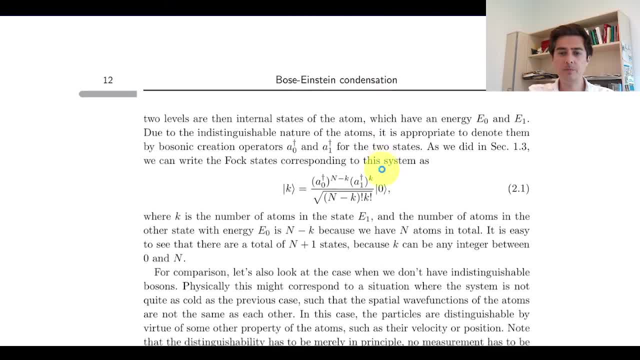 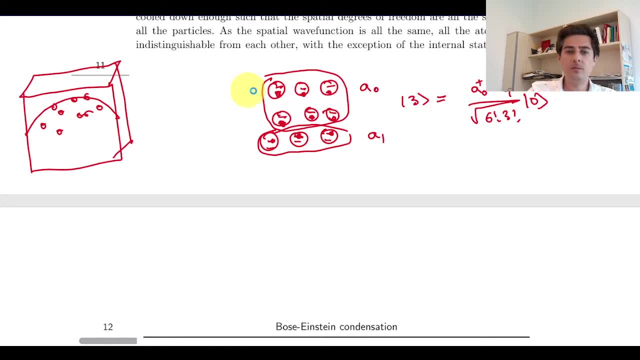 For Distinguishable particles, so I forgot to mention that. So if we write, if we try and write down all the different states of this system, There are a total of only n plus one different states. so this, This K label, just only goes between. 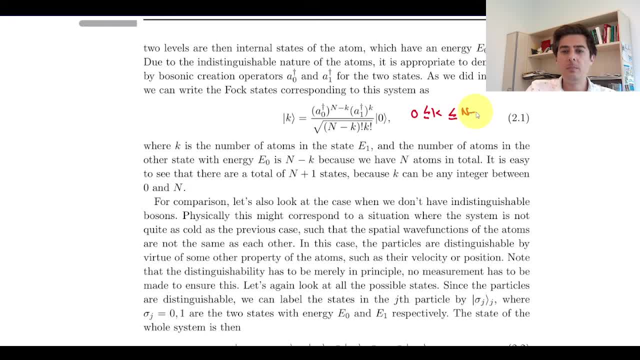 Zero And N plus one. Oh, sorry, N Right. So There are a total of n plus one states, because There's a zero Here involved too. So There's total n plus one states, And Those are the full set of states that. 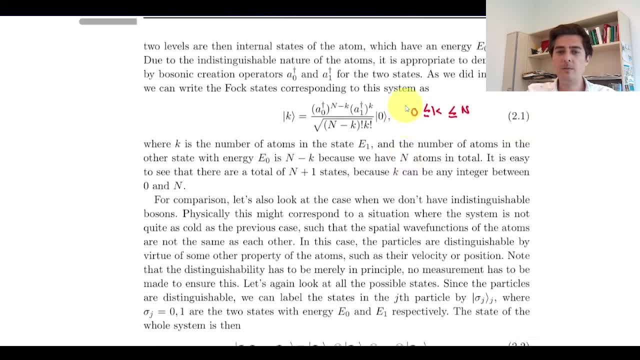 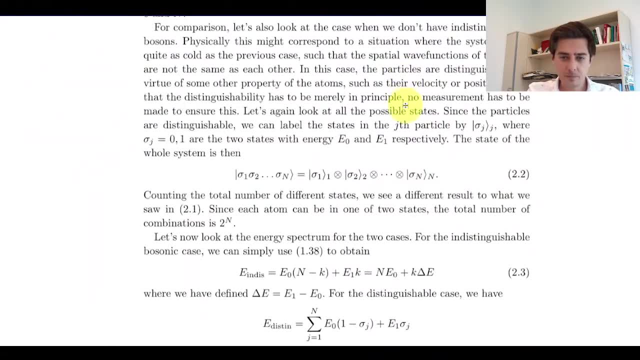 We have for the Indistinguishable case. So What about Distinguishable Particles? Well There, we Sort of have to count The Atoms Bit differently, because Now We can't just sort of group all these guys together and say, well, 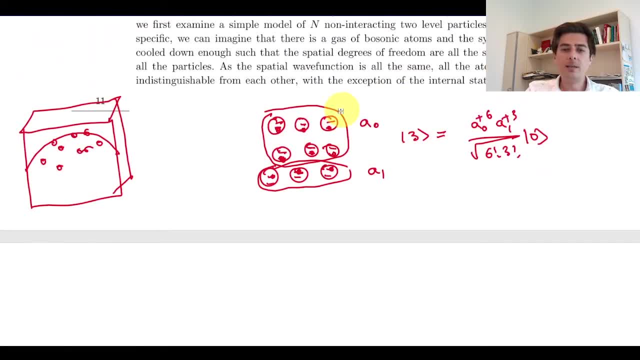 You know You guys are all Indistinguishable, So You know We can't just sort of group all these guys together and say: well, You know, You guys are all Indistinguishable, So You know We can't. 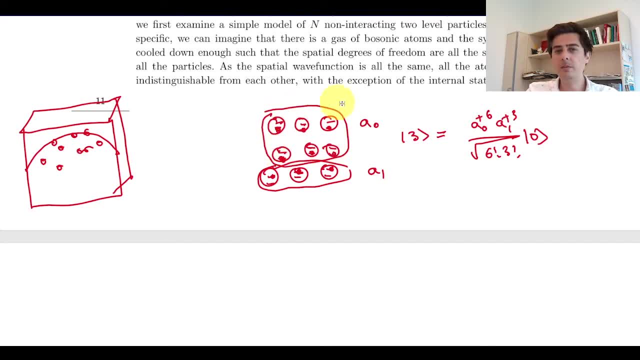 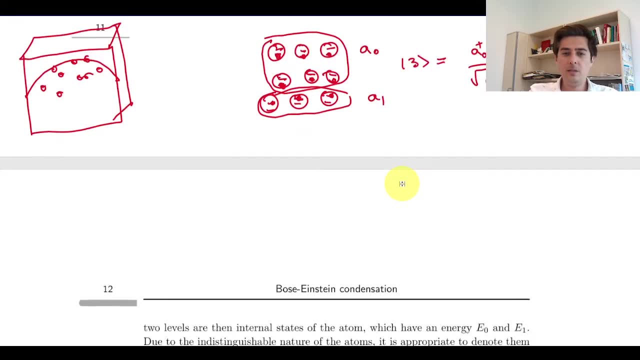 Tell the difference Between You. So The only thing that we can really say is that there's Six of you In this Lower Energy state In the, In the distinguishable case, Of course. So Let me just do a two atom example. 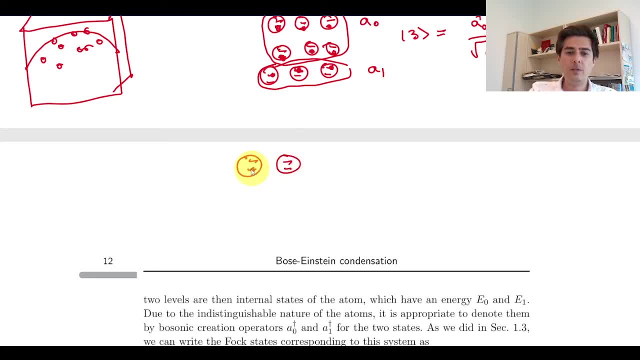 Of course, If, If This guy Is down And this guy's up, You know This Is A different state To Something like this. So Because We Have Labels On These Particular 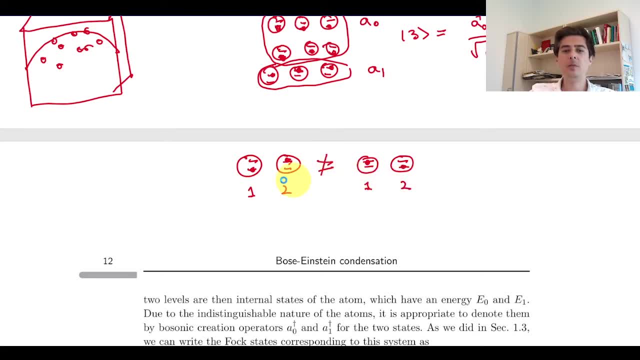 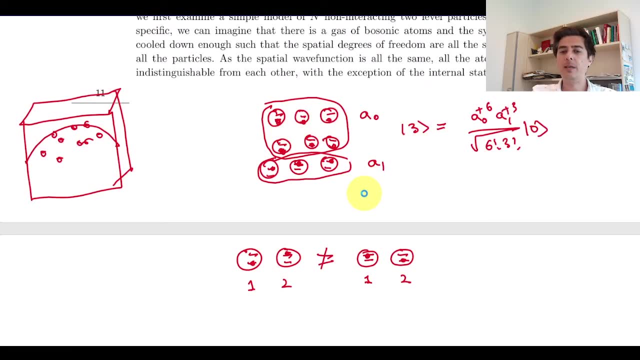 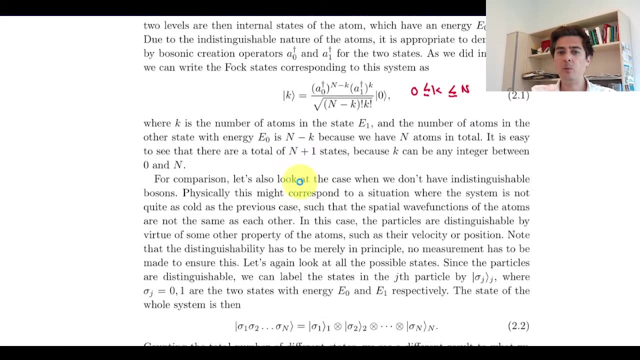 Atoms. So This Is Atom Number One, This Is Atom Number Two. Basically, These Two States Are Different States, Whereas In the Indistinguishable Case Those 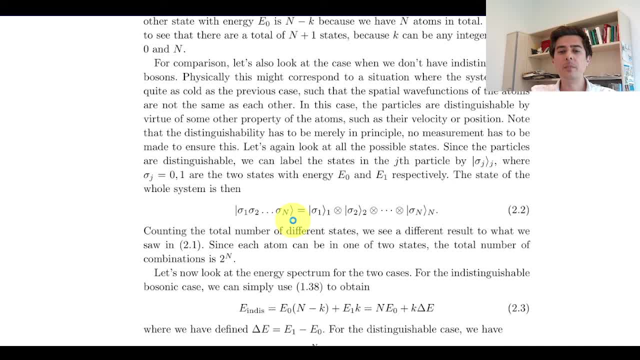 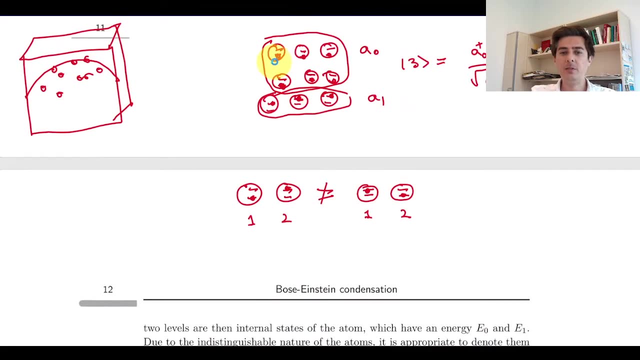 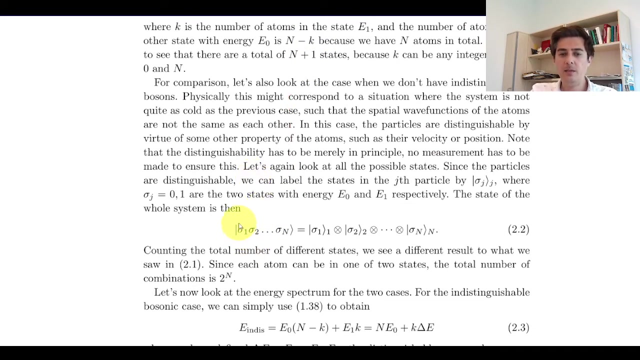 We Are Used To From Classical Physics. In This Case, We Can Actually Simply Enumerate What The State Is Of Each Particular Atom. So There's 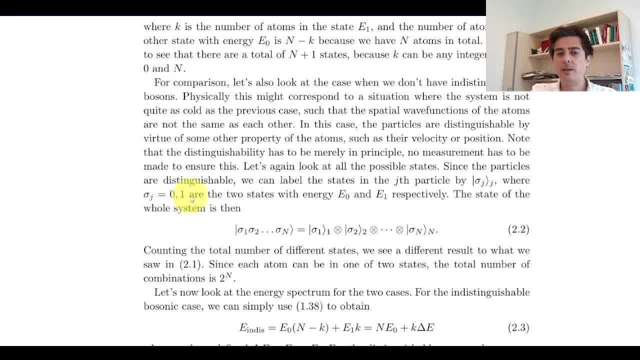 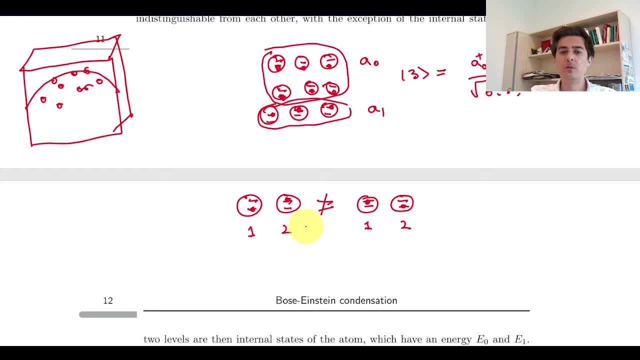 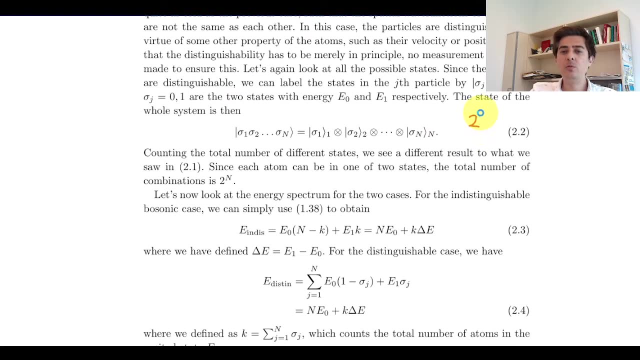 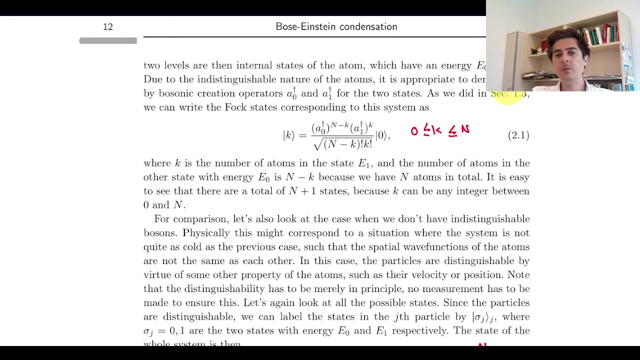 N Atoms. So In This Case There Are Atoms Either In You Know, Zero State, Zero State One, Or Also. So In This Case The 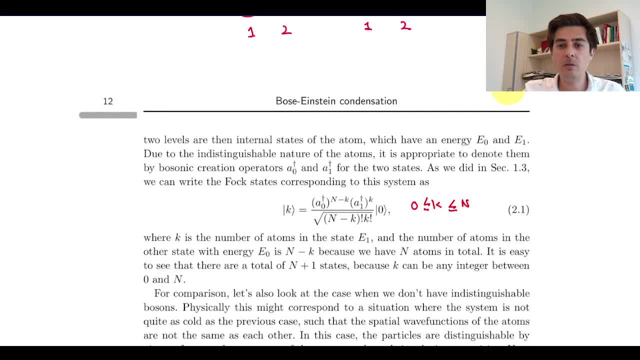 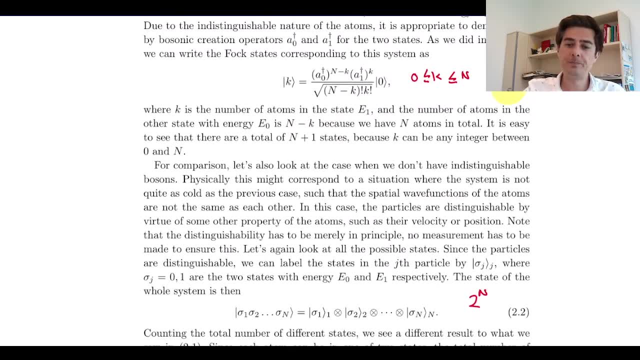 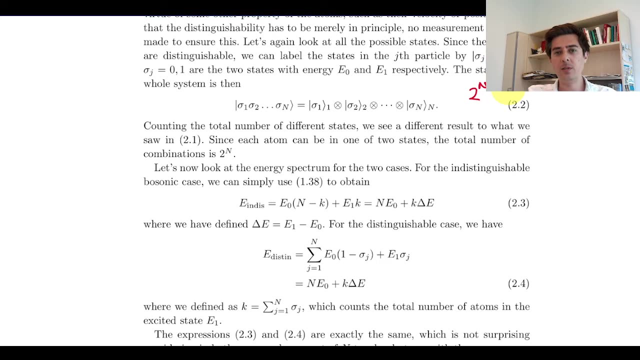 Total Number States Here That We Can Possibly Be A Particle. So This Is Actually Where The Origin Of Thing, This Phenomenon Of Bose, Einstein. 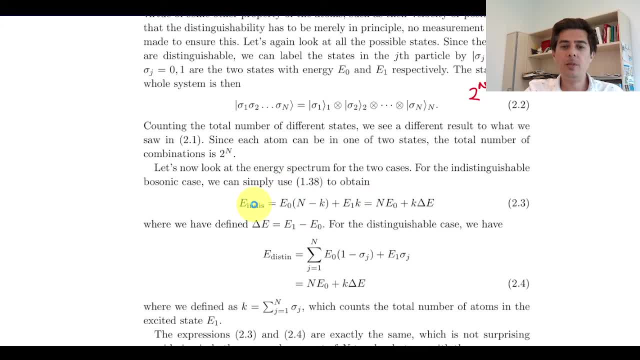 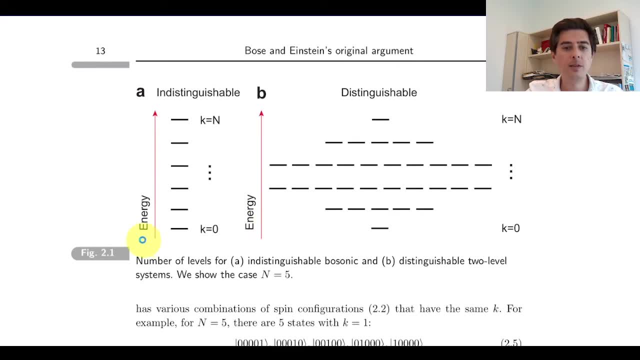 Conversation Will Come From Eventually, So Anyway, So We'll Get To That. So If We Say That Each Atom Say Either For The Distinguishable, 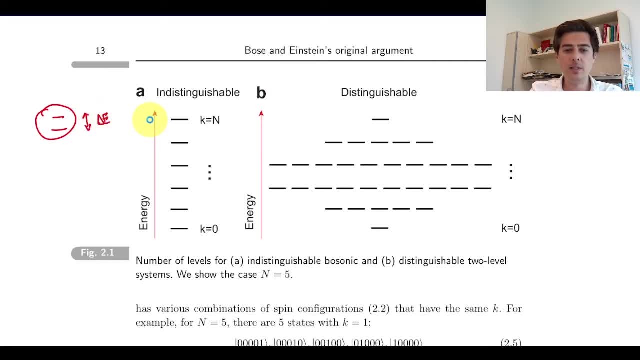 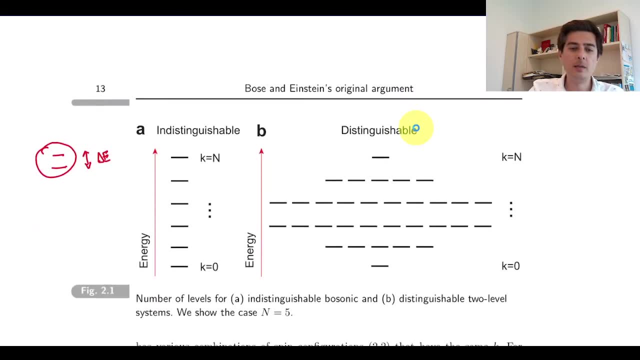 Or Indistinguishable Case. Suppose There's Some Energy. You Know Difference Between These Two Levels Of, Say, Delta, Delta, This Energy Of The Lower Atom. 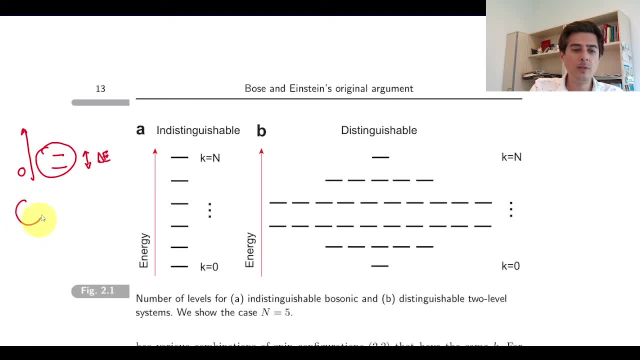 Is Zero, Then In Either Case For The Atoms That Are All In The Zero State. So, For Example, If We Have This, If I 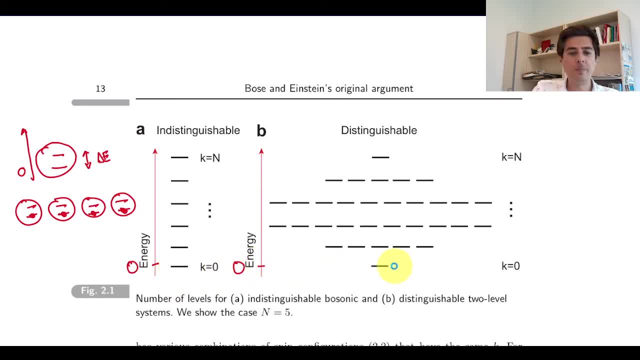 Were To Draw The Scale Here, This, This Energy Here, Would Be Zero. This Would Be The Ground State. Now, If We Have One Atom, That 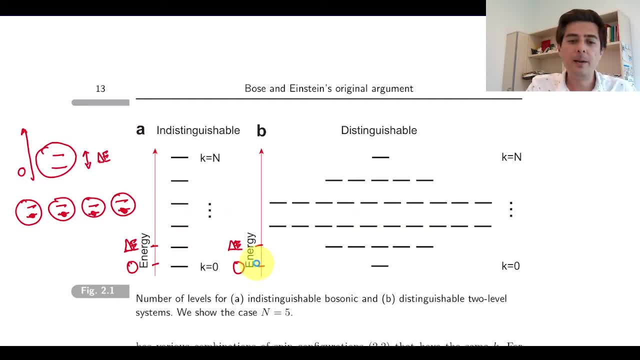 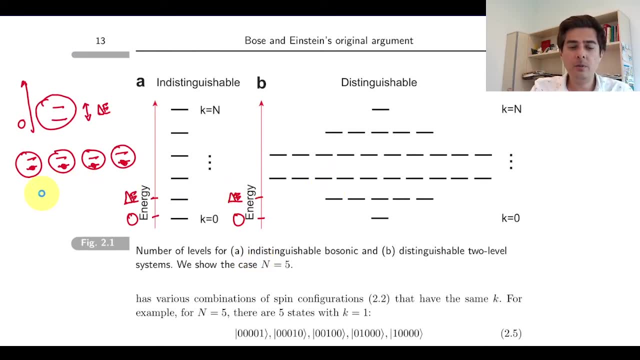 Is One Atom Atom zero. So We Have One Atom That Is Zero. So All Atoms Have One State That Has One Excitation. So The 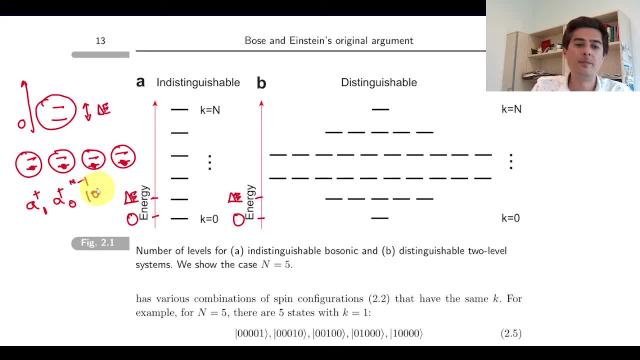 Way That You Write That In, And then if we normalize it, then it would be like so: So in the indistinguishable case that state is exactly that one, But for the distinguishable case there are: for n equals 5,. 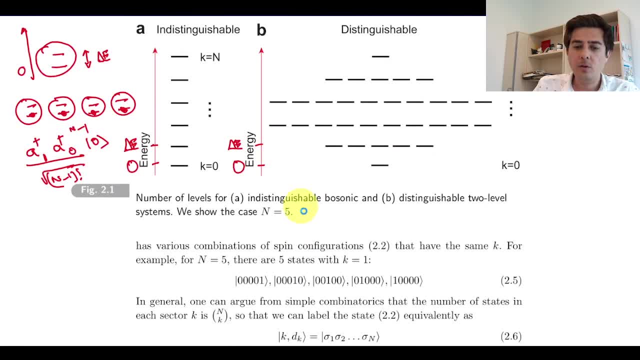 that's the example that I've drawn here. there are five different states which could possibly be the single excited state. So because there's five atoms, it could be any one of those five and that is basically these five states here And then. so I think you get the idea that if you've got two excited states, 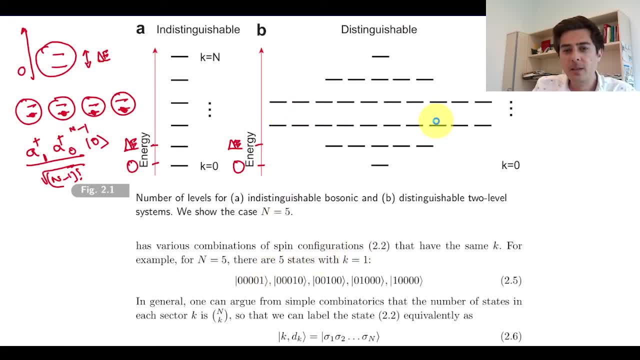 then this is a sort of a combinatorial thing. So then these are all the different states that you would get with, say, two excitations within five atoms. So I think this is 10.. So because eventually this is a combinatorial, where for each level 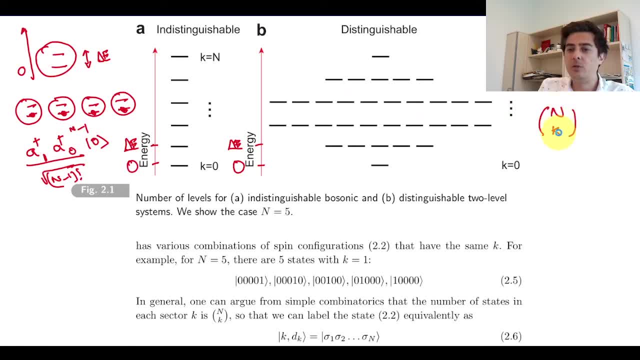 there are n choose k number of states that satisfy this right. So the spectrum in terms of the energies is identical, right. So this top state, for example, would be n, delta e, for either one And in each case. 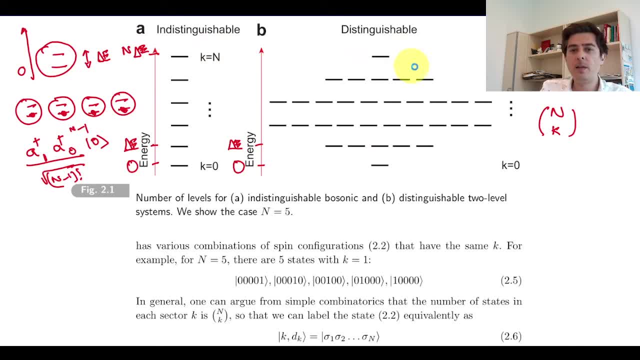 these extremal states. there's only one state like that, But then, for the distinguishable case, there's just a lot more states here that are in the middle. And if you know what a binomial distribution looks like, if we plot the binomial distribution, 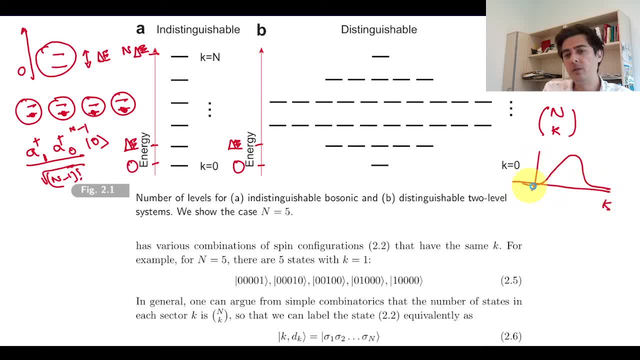 then this always looks something like a Gaussian right. So there's a huge number of states right in the middle here where k would be roughly n over 2. And there's a huge number, a number of these ones, because this would involve 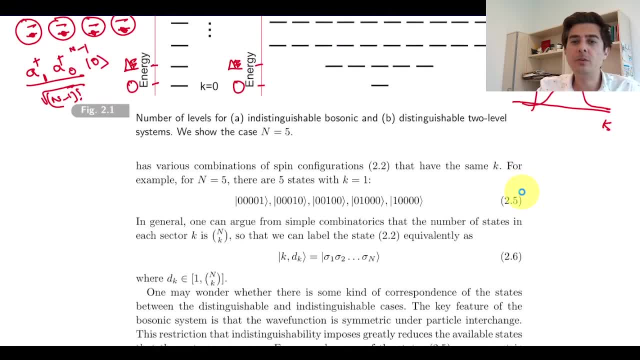 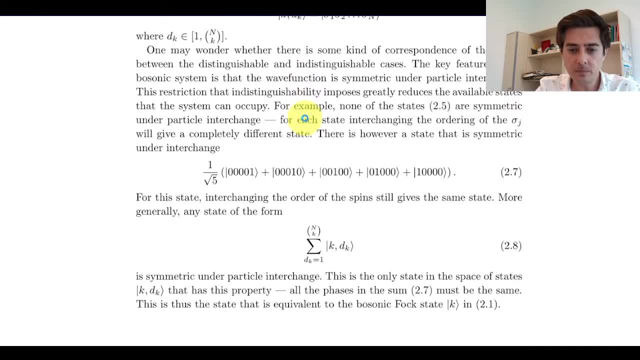 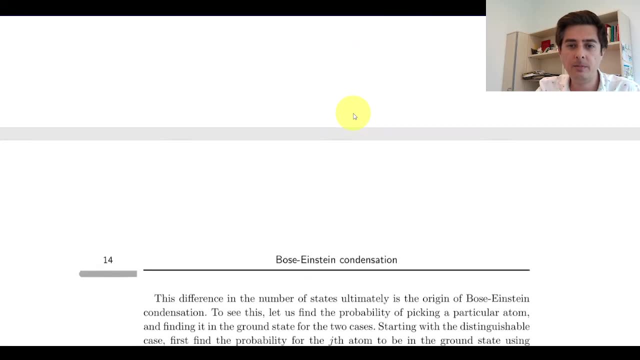 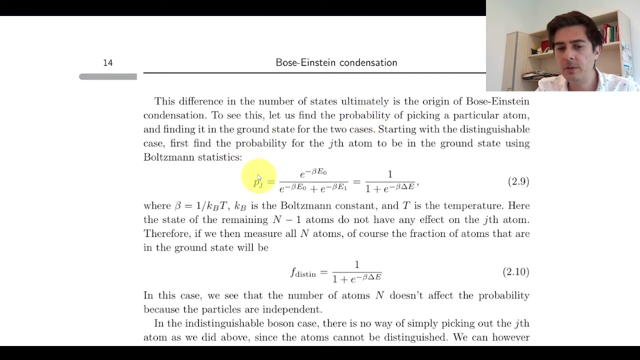 you know factorials and so forth. OK, so ultimately this difference in the spectrum is going to make a big difference. So let me sort of skip one part here, maybe come back to it later and give you the basic argument. So now let's consider this. 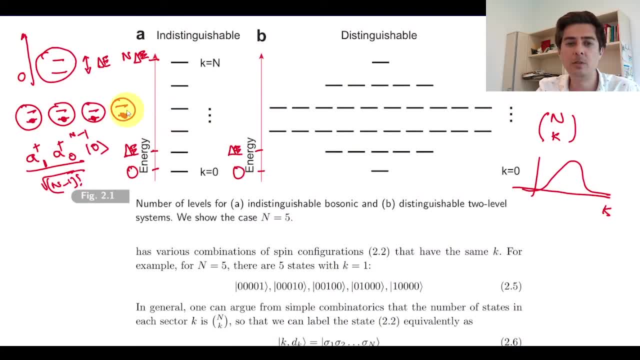 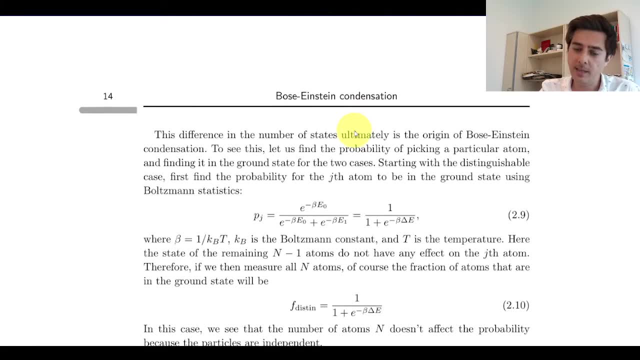 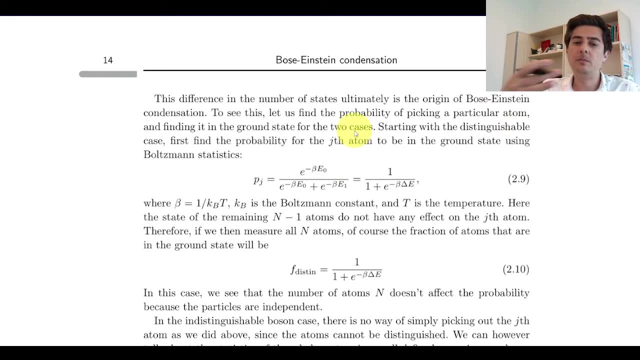 system. So you know you have either an indistinguishable or distinguishable system And there are some temperature T right. So in either way or in either case they follow kind of Boltzmann statistics, because you know Boltzmann statistics simply says that if you've got an energy 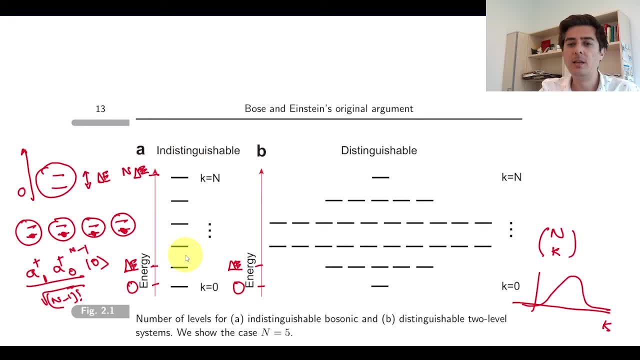 you know energy spectrum such as this, then the states will follow and the probability of following of a particular state being occupied is going to be, you know, E n over k, B, k, B, T, right. So whatever the energy of that state is, 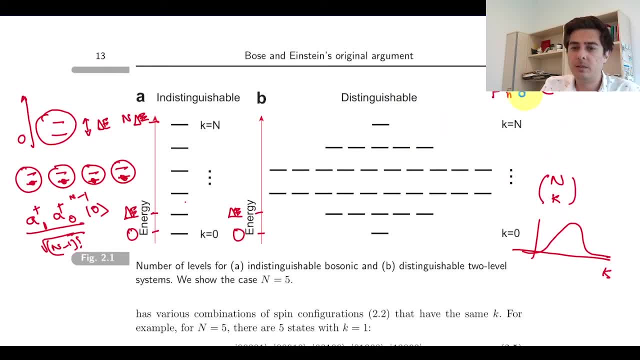 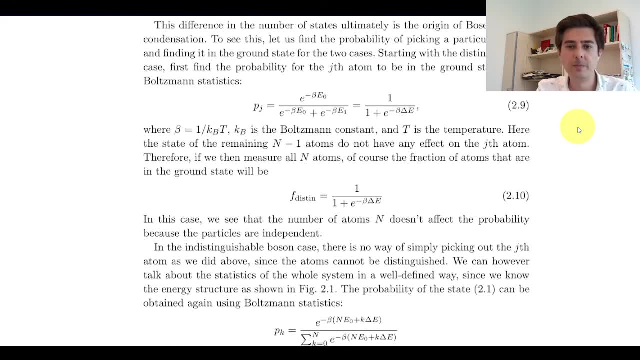 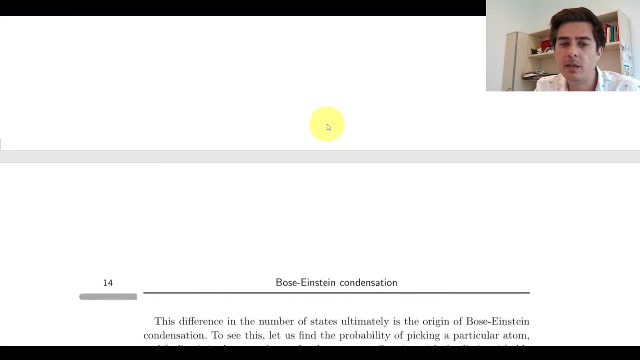 divided by k, B, T, right, And then OK, that's. there would be some normalization factor, which we normally call the partition factor. And so if we were to try and say OK, or try and calculate, let's say we've got, you know, a bunch of atoms and 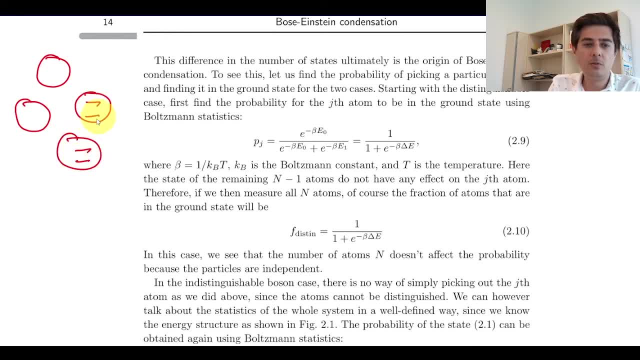 they're all at some temperature. you know this whole ensemble is at some temperature T, So obviously some of these ones, as long as it's not like zero temperature, some of these ones might be excited and some of these ones might be in the ground state right. 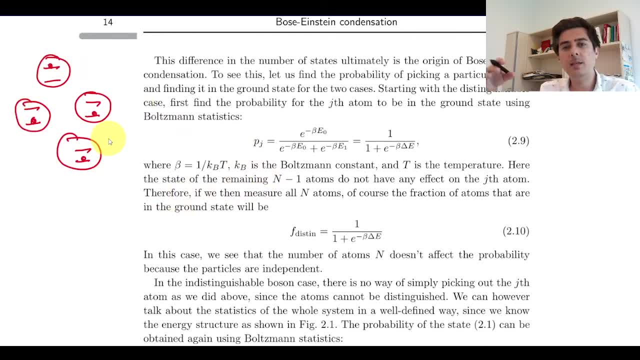 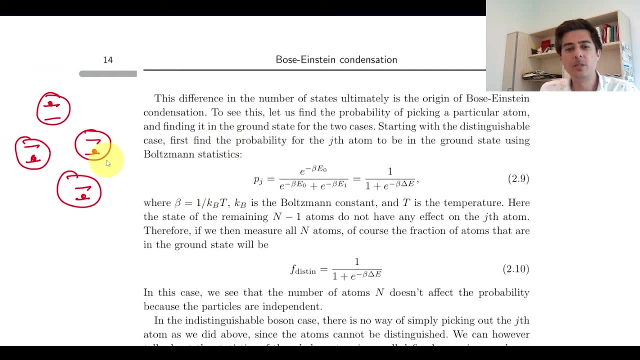 So because these are actually completely independent atoms, you know so, because it's, you can kind of break this system down into individual components. There's actually a simple way of calculating the probability of finding how many atoms are going to be, say, in the ground state. 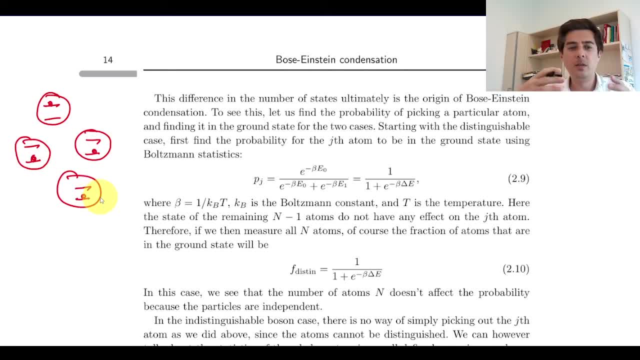 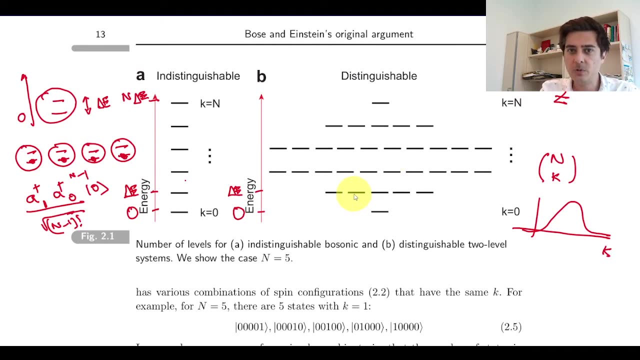 And it's simply that you you look at the system just on an individual basis and basically because you know we can treat this whole thing as an ensemble, and then do the calculation kind of the hard way, where we look at this entire spectrum, calculate the Boltzmann distribution for that and then work out the probability. 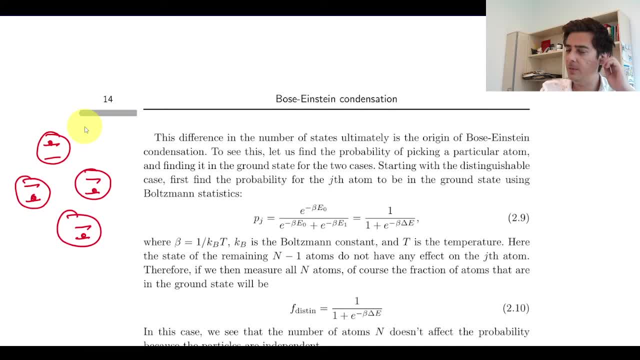 of how many of these are going to be in the ground state, How many are going to be excited state. So we could do it like that, but we actually can get exactly the same answer much simpler way by basically saying that: well, OK. 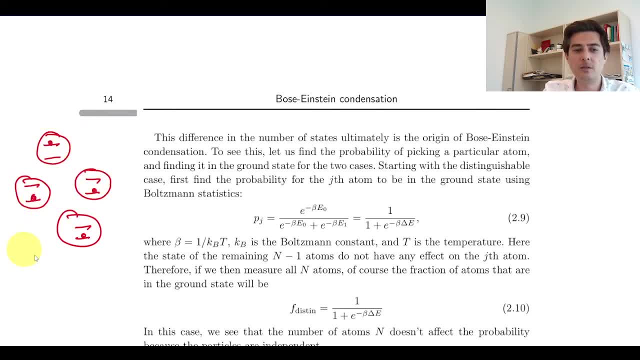 these are basically independent, right? So even though we're going to look at this whole thing as a whole, let's just look at like one atom and then see what it does. And because these are all independent, actually it still holds for the whole. 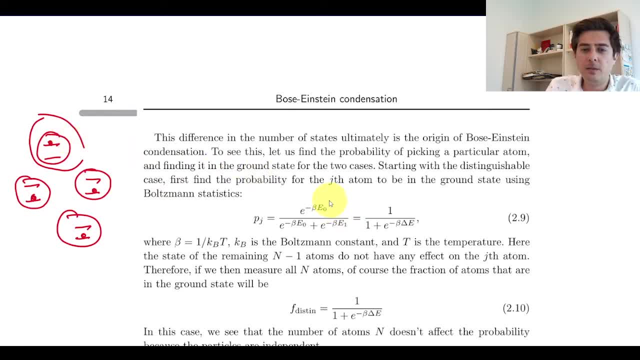 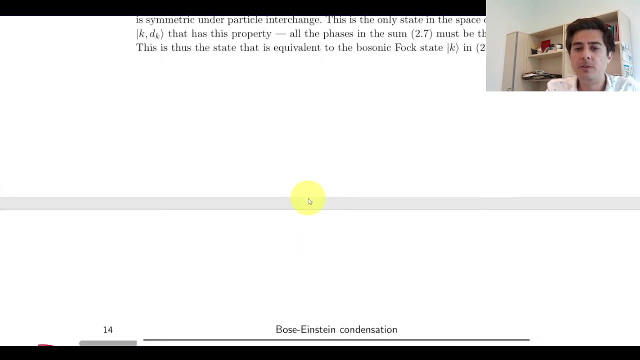 system right. So for a single atom we can easily calculate the probability of it being the ground state, because so it's this Boltzmann factor. The beta is of course one over KBT, And then you divide by the partition function, which, for a single qubit, 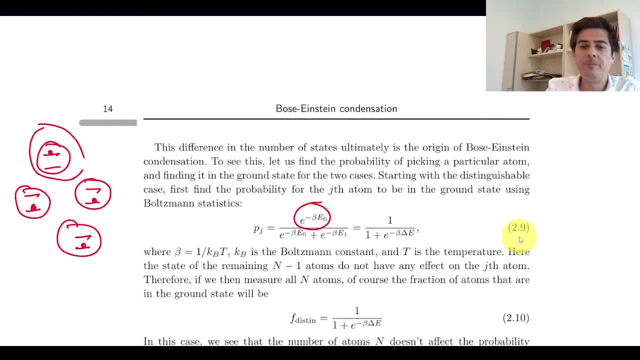 So that's that Z factor which I was talking about, which is for a single qubit. it's just simply the probability Boltzmann factor sum of each of those two states. So this partition function is super easy in the case of a single qubit. 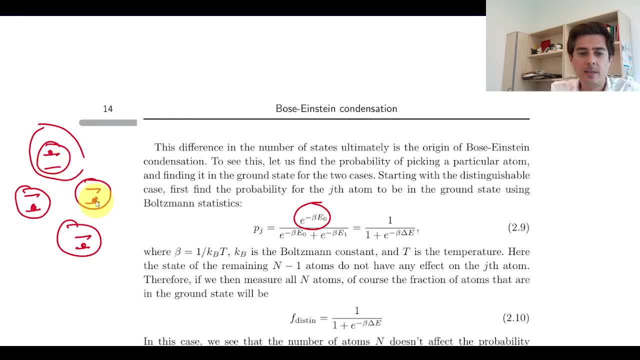 And so the probability of it being in the ground state, like like this particular atom, is simply equal to that, And this delta E is just defined as this delta E here is E1 minus E0.. So that's just a separation between these guys. 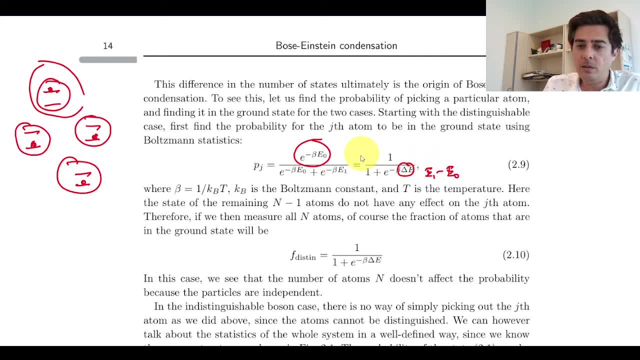 So so the probability is equal to this thing And and the the key thing to notice here is that, because these are all independent, this is actually independent of N Independent, So it doesn't really matter how big your ensemble is, because these are not really. 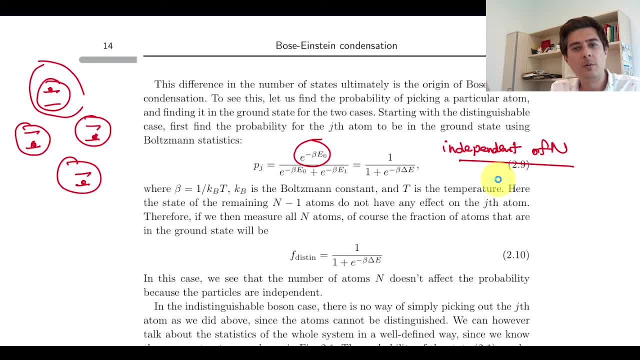 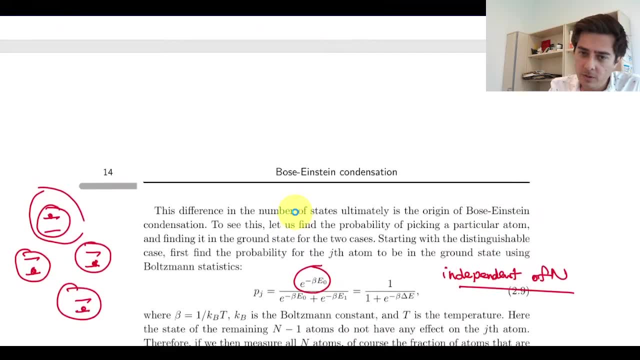 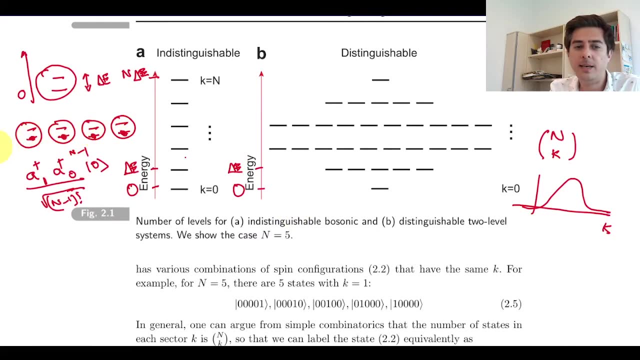 interacting with each other. they, it doesn't really matter what it is, But in the indistinguishable case, actually, it does make a difference. because you can't really, In this situation where we are treating these atoms as indistinguishable, we can't just sort of focus in on one atom and then forget about the rest. 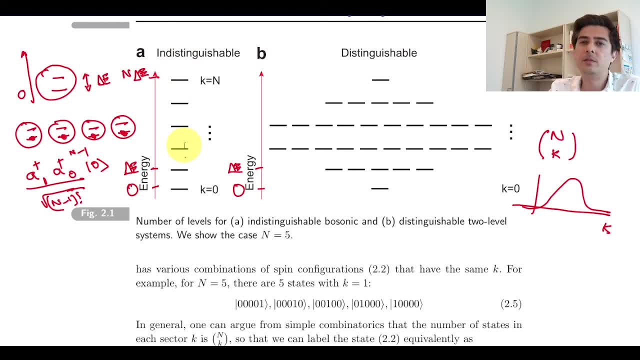 because really the spectrum and the set of states that you have with an indistinguishable bosonic system are kind of all it's kind of linked to each other And the properties of one are not really kind of separable from from the remaining of them. 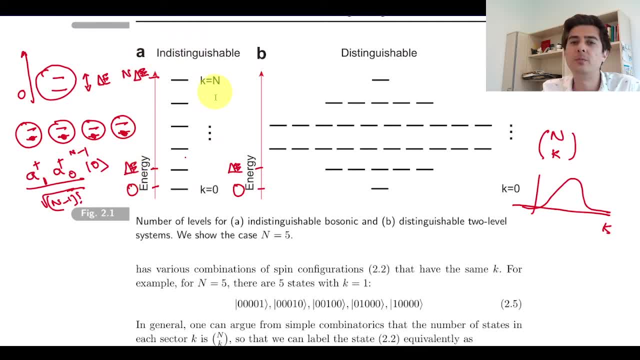 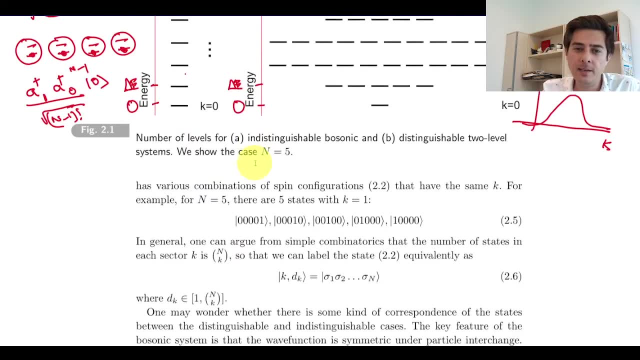 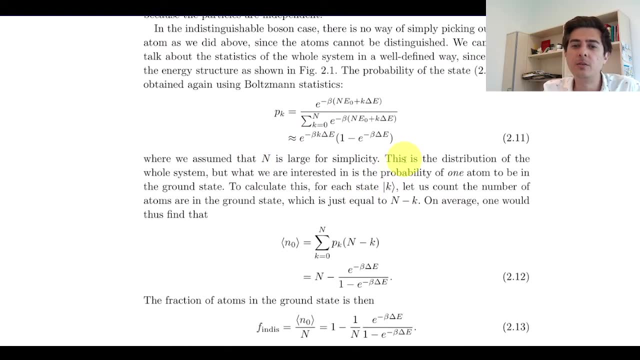 So in this case we really have to look at the full system as a whole and then calculate the Boltzmann probability of the spectrum and then deduce what the probability is of finding each atom in the ground state. OK, so the way that you do that calculation is a little bit different in this case. 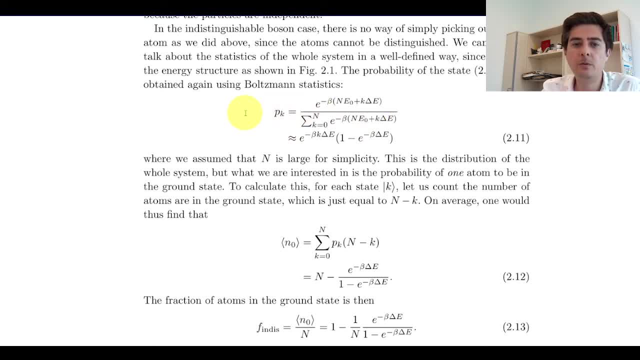 So in this case, um the probability, what you do here is you say, OK, well, the energy spectrum looks like that, So that's just just what I have on the previous page. And then the energy on on the nth level is simply n. 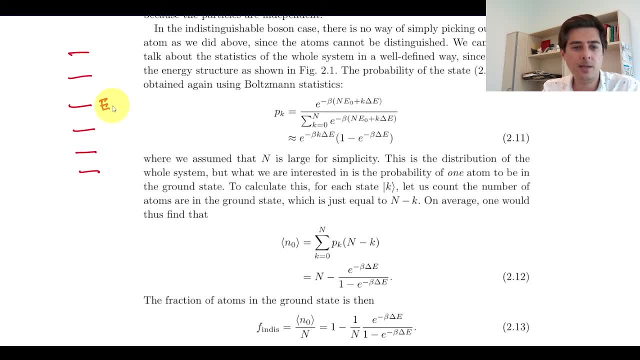 Oh sorry, I used k, So let's go back. OK, So the energy of the kth level is k times delta E, because you know each one of these ones is delta E. And then let's say: let's say that, OK. for some reason I didn't start at zero here. 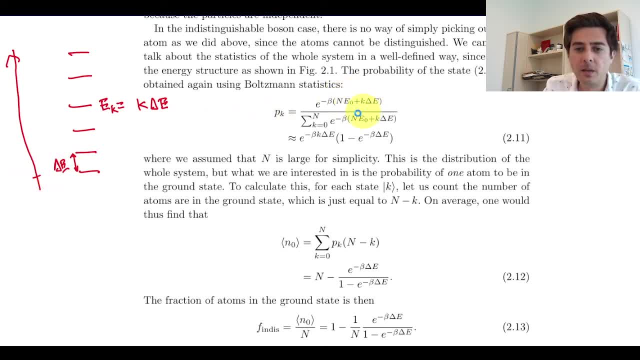 But if I started at zero, these factors would be not there. In fact, maybe if you do that it's a bit simpler. So let's just say that. well, OK, just so that it matches with this equation. the energy of the ground state is E zero. 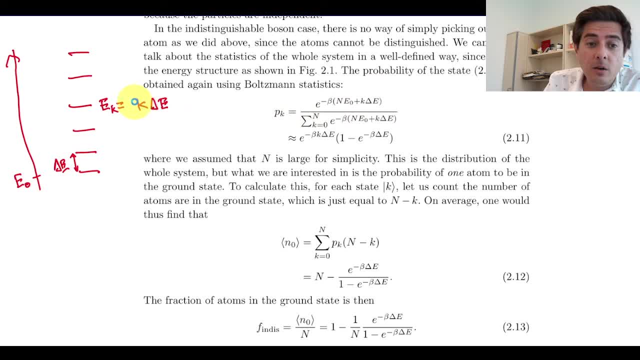 And so the energy of this state would be kth, delta E above whatever that is, And so for n particles that would be n E zero. So in other words, it's like we've got n particles in the ground state, but then we've lifted k of them out of it. 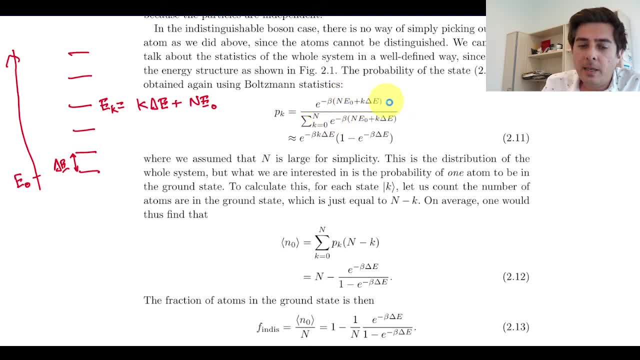 OK, so that's the energy level of that particular state, And then to find the partition function, then you know we have to sum over the probabilities of every possible state, And so that's why there's a sum here from k, zero to n. 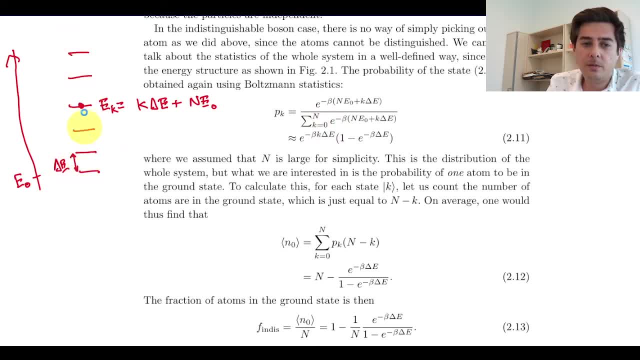 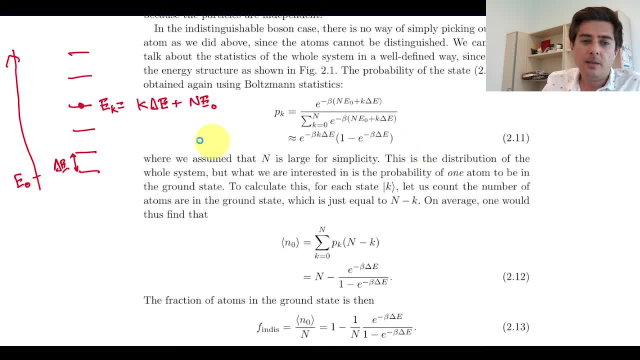 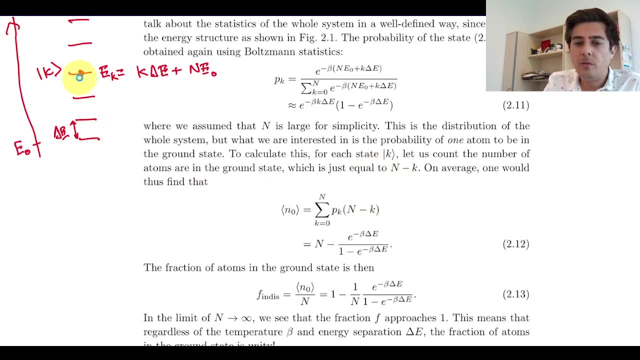 And so the probability is equal to this, And so that's the statistical probability of the state being in this kth level. And then what we're going to do is we're going to calculate So for the average of the whole system, because, you know, sometimes it's in this state. 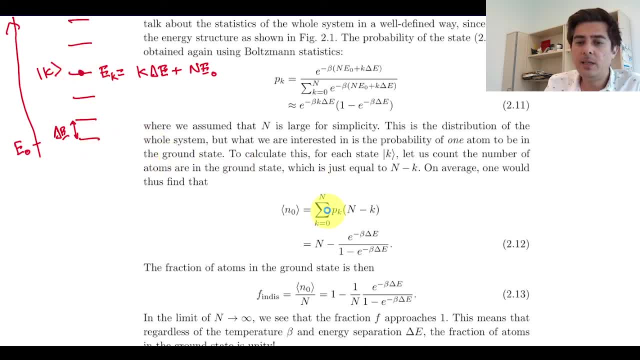 sometimes it's in a different state and so forth, And let's calculate the number of atoms that are in the ground state. So this n zero operator I'm going to define as being a dagger zero, a zero. So that's this, that's the 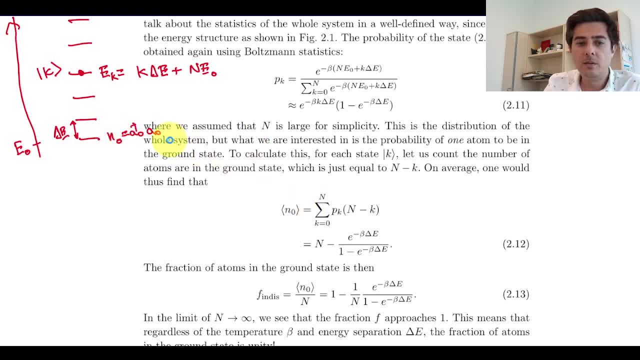 number of atoms that are in the total number of atoms that are in the ground state. So, for example, this would count. So if you've got a bunch of atoms here, say this is your state and say you had two atoms here in the ground state and 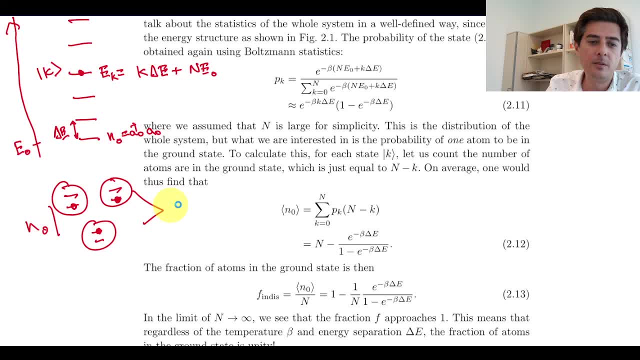 then one atom in the excited state. So the operator n zero would basically just count two atoms that are in the ground state. So for example, this would return two for this particular state. OK, so this counts the number of atoms that are in the 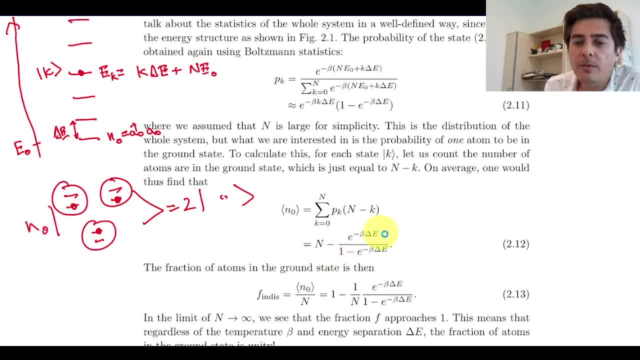 in the ground state, And if we take an average over all the different states in the spectrum, then this time we actually get an answer that looks like this: And so here, what's going to happen is that it's going to be n minus this. 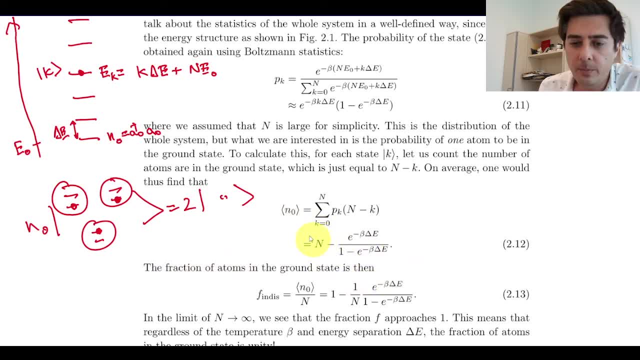 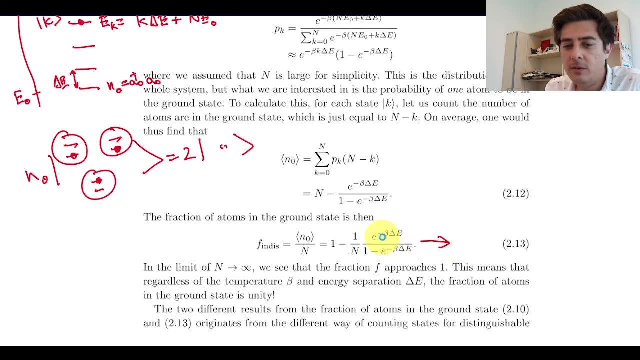 And then. so the fraction of atoms in the ground state would be simply this divided by n, And then now we actually get something with an n dependence, And if we look at the case where n is actually large, then actually this thing. So you know, let's consider a fixed. 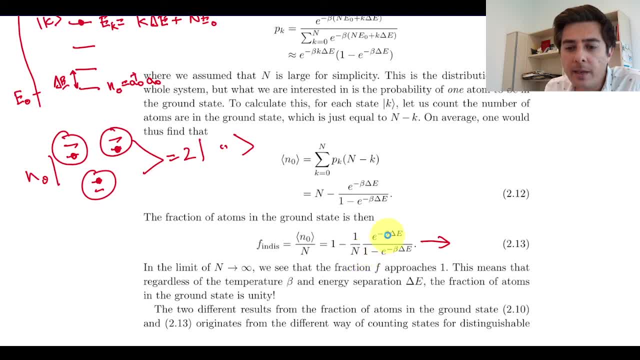 temperature, fixed energy, so forth. then this will be just some constant factor, But then this is a diminishing factor, So one over n is going to go to something very small, regardless of what this is, And so actually this is going to approach one. 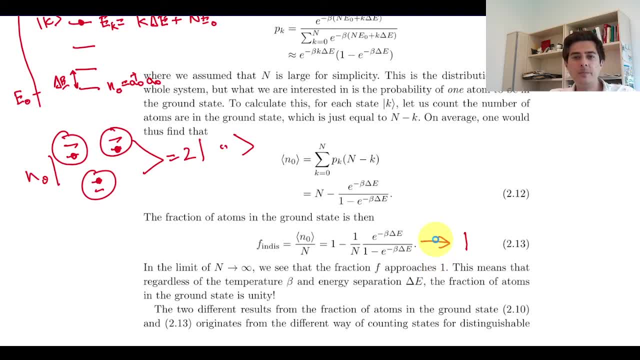 So this is, this is very interesting because just because we counted things differently, of being either distinguishable or indistinguishable, we get an entirely different result for the number of atoms that are going to be in this lower energy state. And you know, maybe 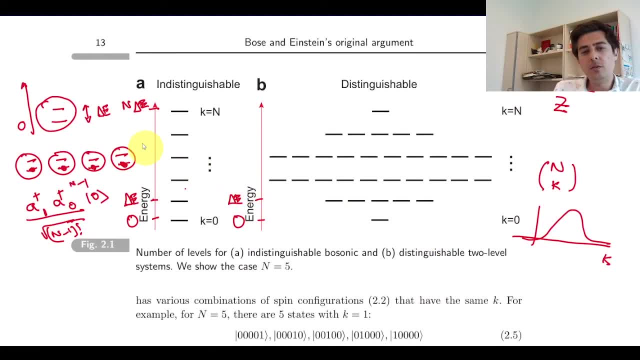 sort of a casual way to understand this is that, you know, because the spectrum is is quite different, this Boltzmann factor is always an exponential. So if we kind of put our head on their side and then look at the exponential distribution, whoops, I don't know what happened there. 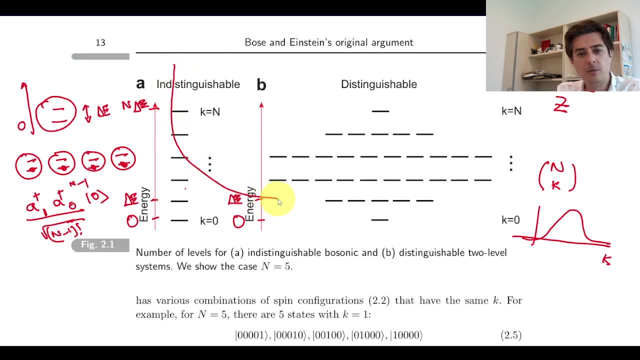 I'll do that again. So exponential distribution goes up like this. So here it's kind of natural to expect that there's going to be a high probability of states in this lower state. But we also have the same exponential factor over here. But then we have this very strong weighting towards the middle here. 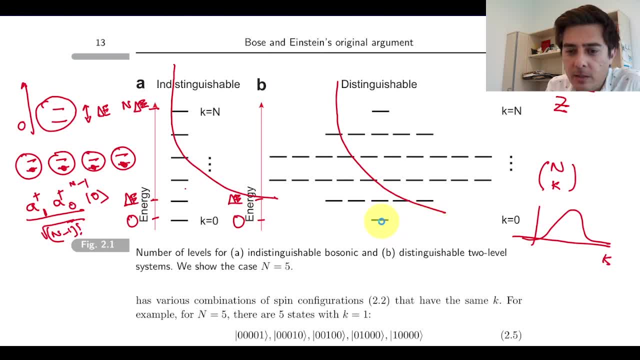 So, even though this state by itself is way more probable than any of these other ones, But then because there's so many of these ones, all these ones add up and it actually makes it kind of balances out, this exponential right. So, because you have, as I said, this binomial factor, 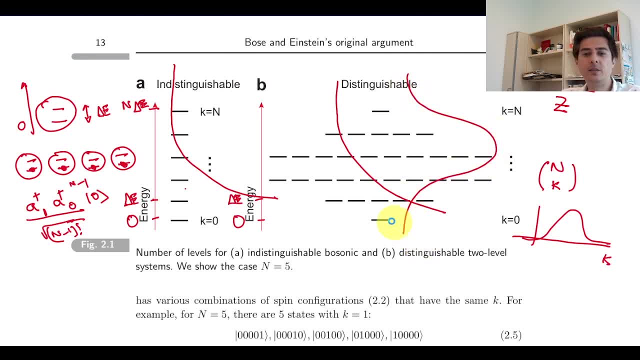 which, in terms of sort of the number of states, is weighted like this. So, even though this is big here, this is actually small, And then, you know, binomial is actually quite big here, where this is actually a bit smaller and kind of. 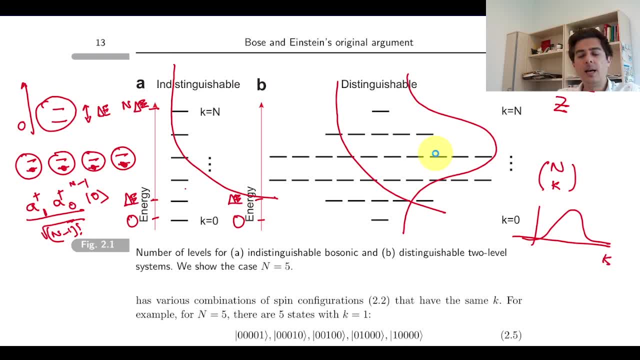 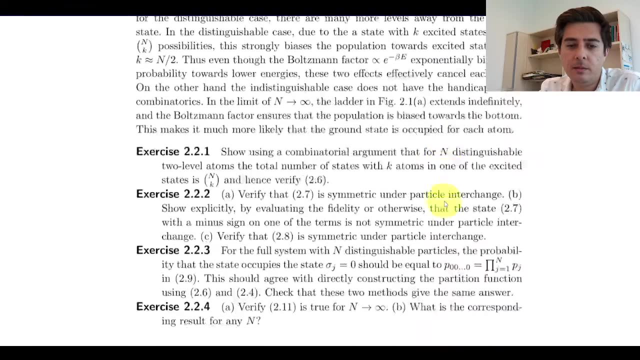 sort of cancels each other out, you know, in a way. So this is why it makes a big difference of whether things are indistinguishable or distinguishable, And OK, and I think maybe we might leave it there because I don't want to start going through all these exercises. 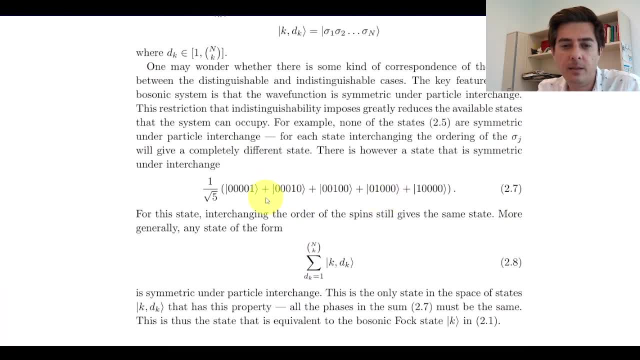 And also we. I missed a small point here regarding the symmetry, But I think we can cover that in the next lecture. So so, if you have any questions on on this topic- I hope this was a bit helpful for you to understand how Bose-Einstein condensation occurs- and have any questions.